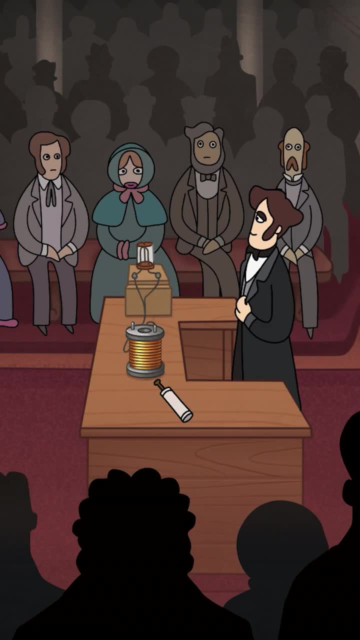 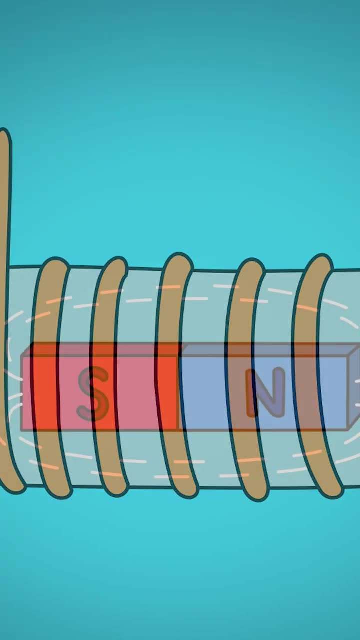 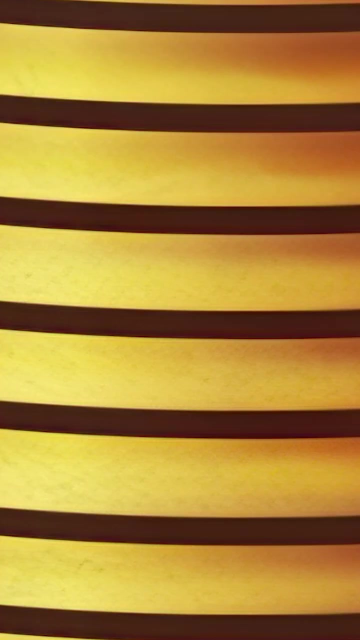 In 1831, Faraday conducted a similar experiment for the first time. For this we need a coil, copper wire and a magnet. We insert the magnet in a coil wound with copper, we move the magnet inside and in each coil of copper a voltage of 0.01 volts is generated. 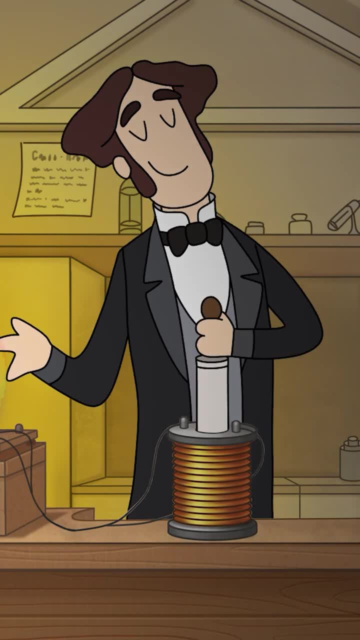 But due to the large number of turns, everything is working just fine. 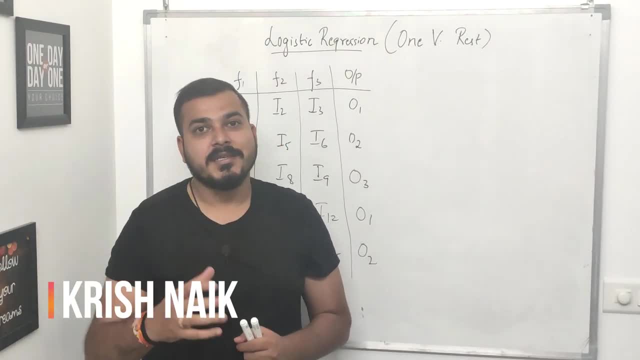 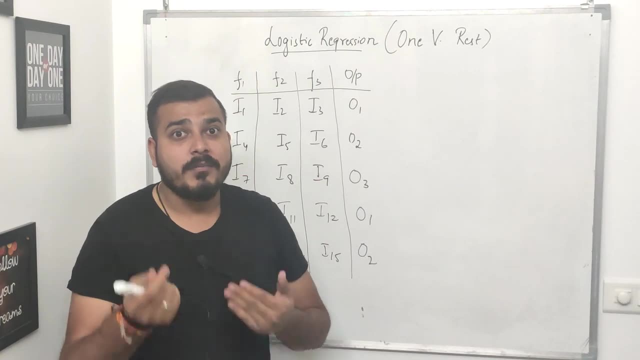 Hello all my name is Krishna and welcome to my YouTube channel. So, guys, today we'll be discussing about the logistic regression, part 3, and here we are actually going to discuss how we can solve a multi-class classification problem with the help of logistic regression. Now, probably you may have 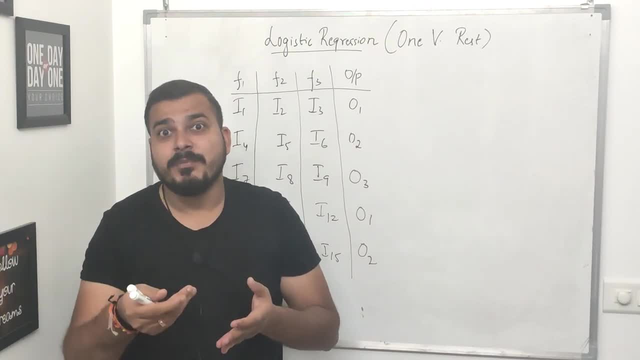 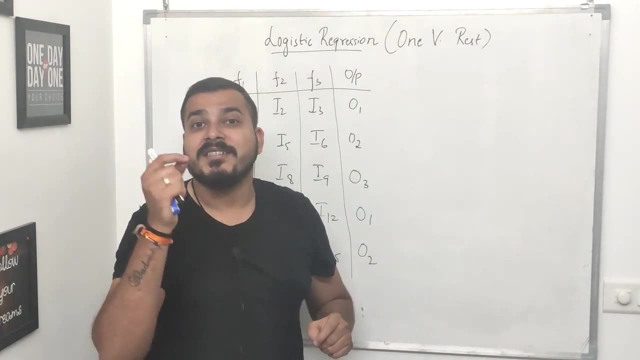 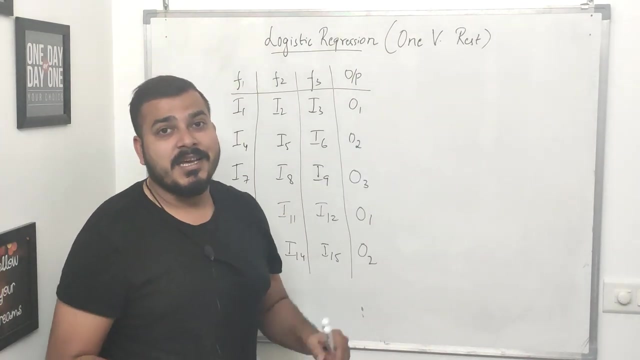 heard only solving binary problem statement, binary classification problem statement with the help of logistic regression. but now, today, in this particular video, we'll try to understand one concept which is called as one versus rest, or it is also called as one versus all. How does it actually work Now, if I'm talking about one versus rest in logistic regression? we know that we. 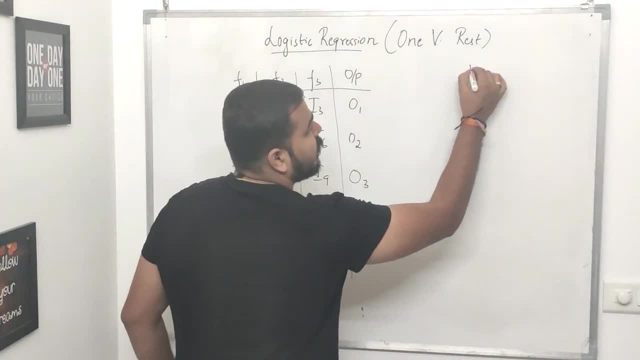 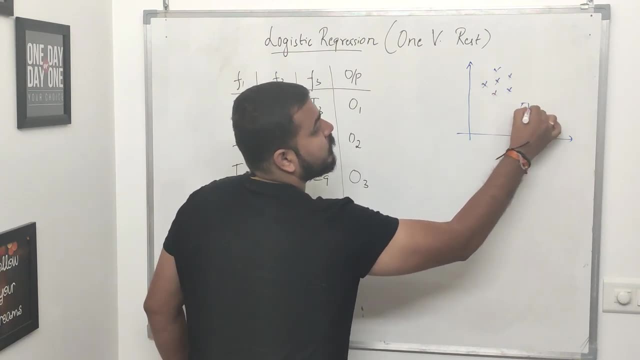 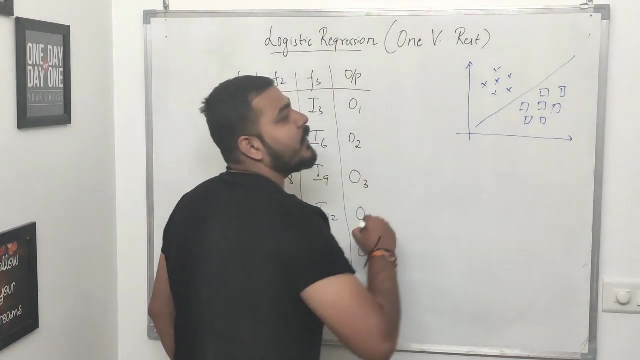 actually try to solve a binary classification problem. Now, suppose if I have a problem statement over here and suppose if I have two categories, which looks like this, right, so this is my two classes now in order to solve this particular binary classification problem, I try to draw a best fit line in between them and then we try to solve this particular problem, right. 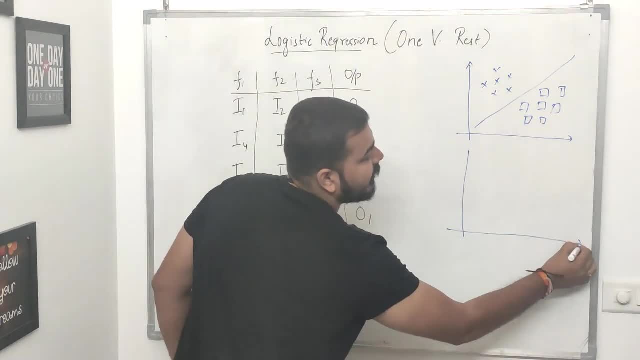 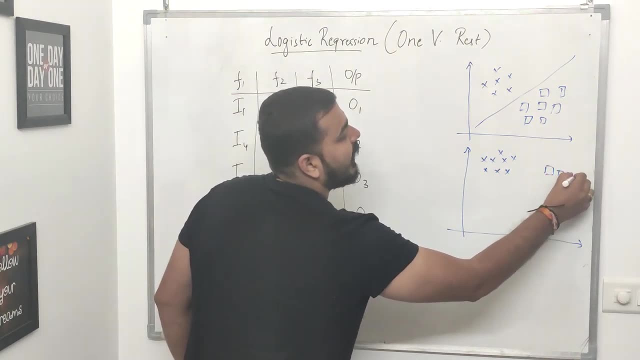 Now what if? if my output categories are multiple categories like this? suppose I have over here as star, suppose this is one of the things, this is my another classification category, right, and suppose this is my another category. now suppose if I have this kind of solved problem statement can we solve with the help of logistic.